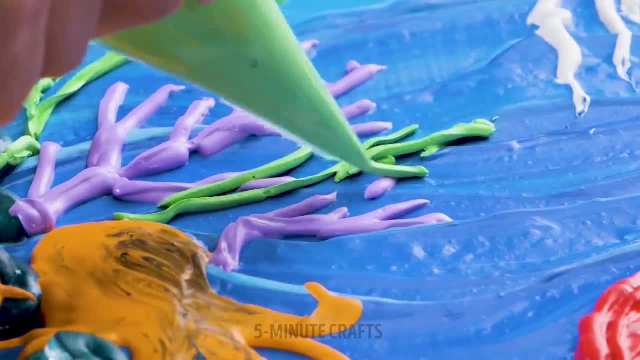 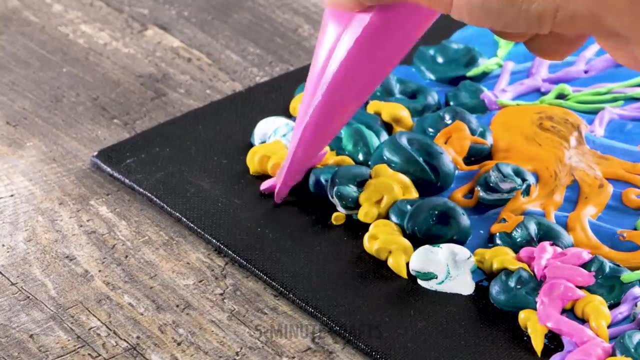 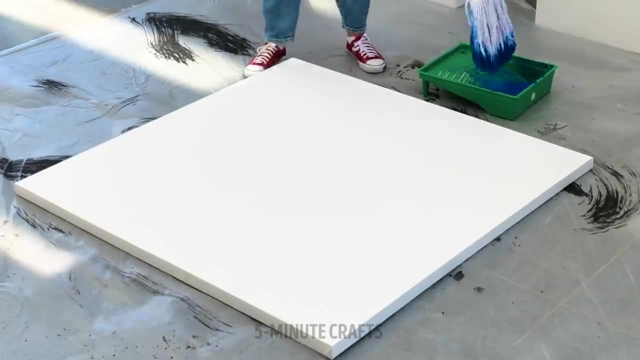 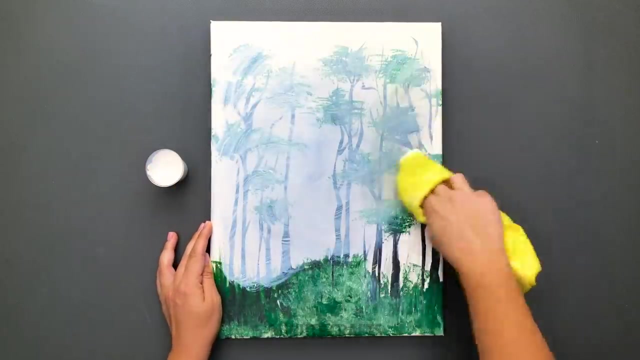 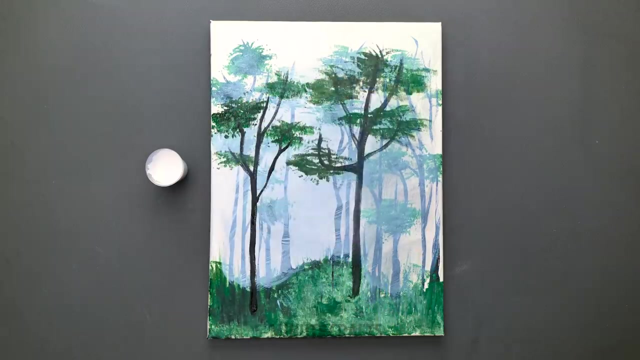 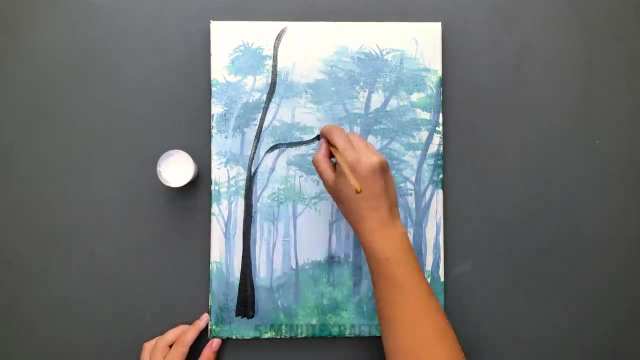 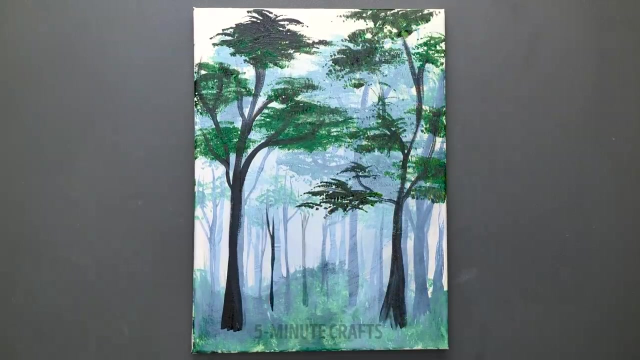 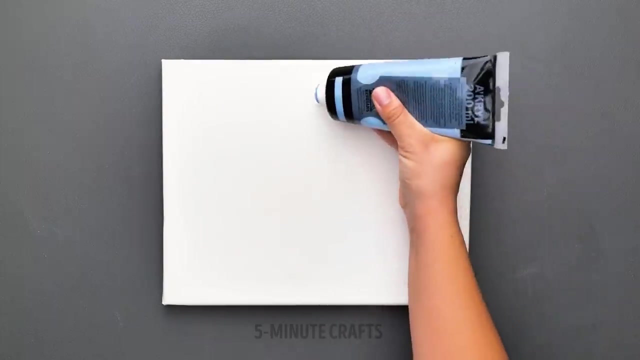 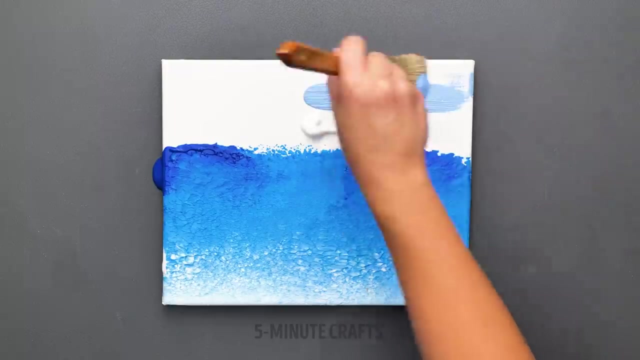 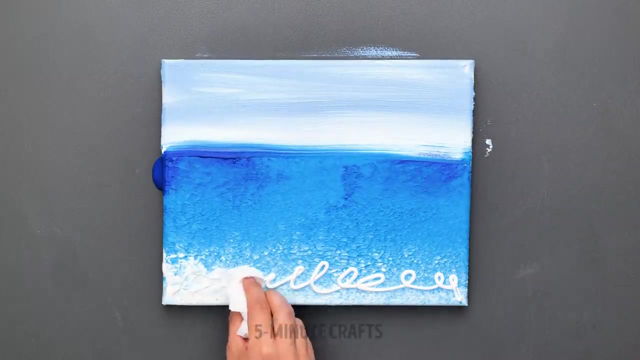 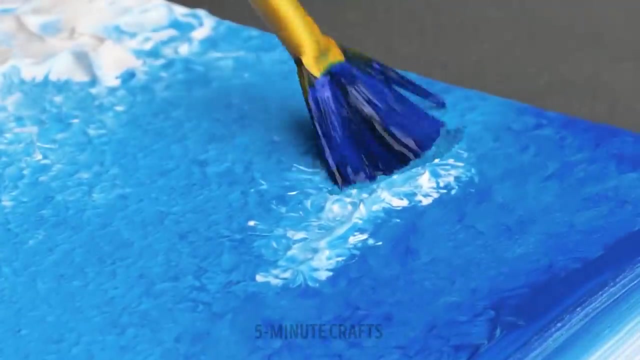 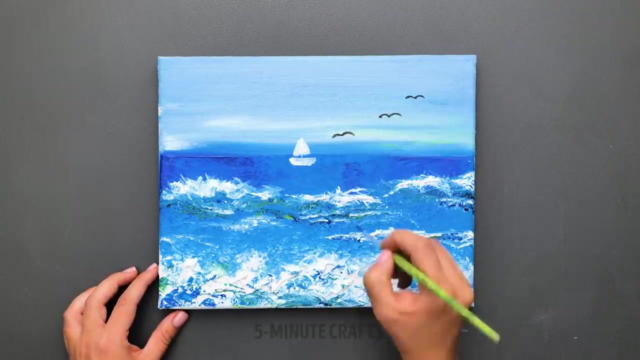 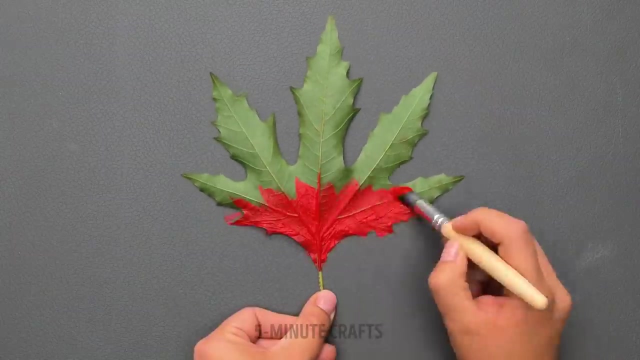 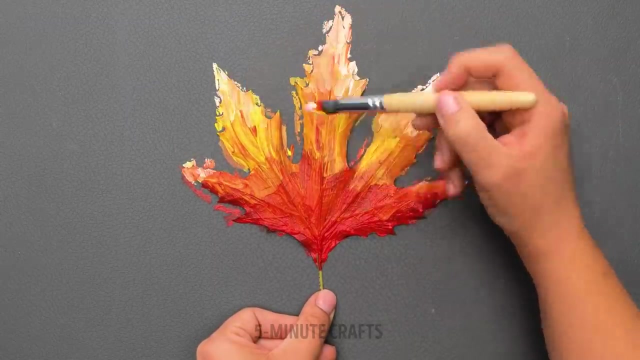 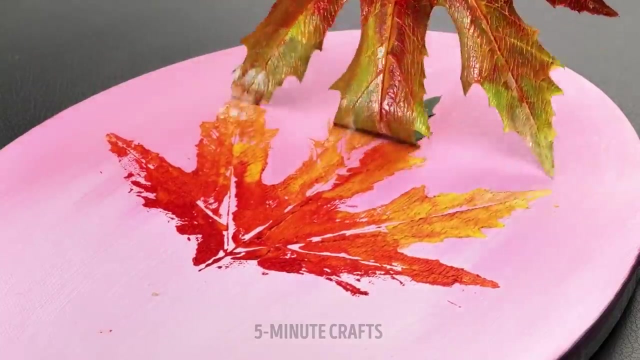 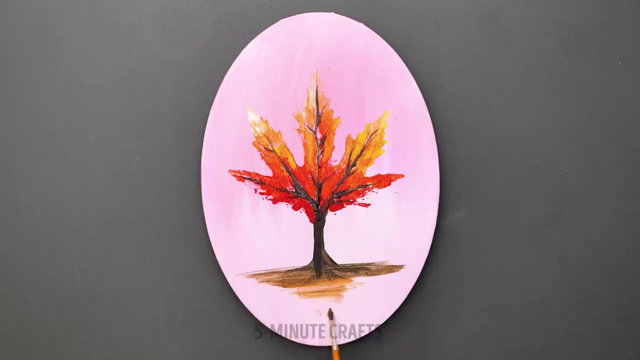 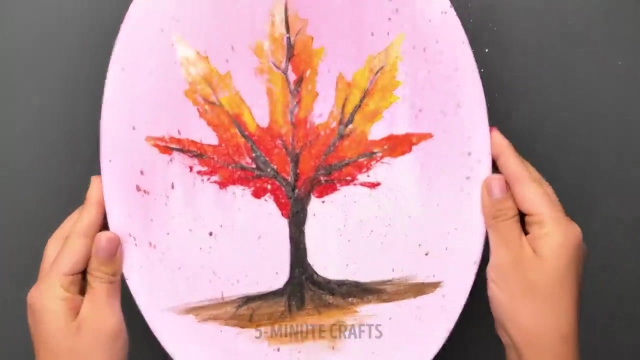 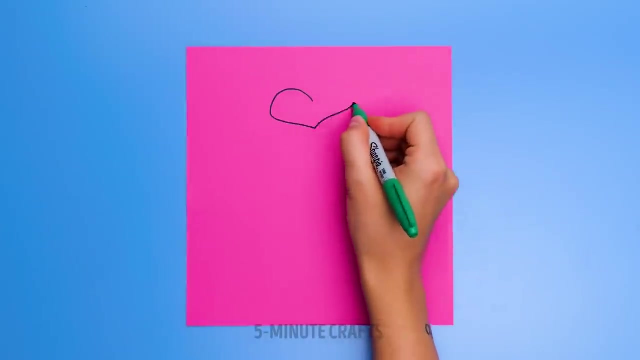 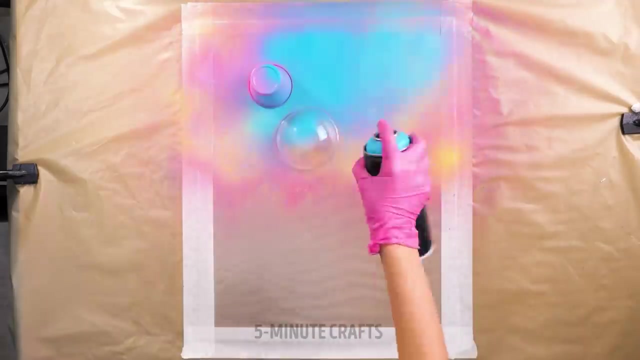 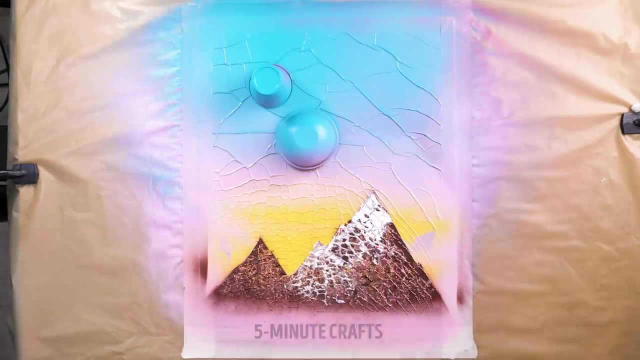 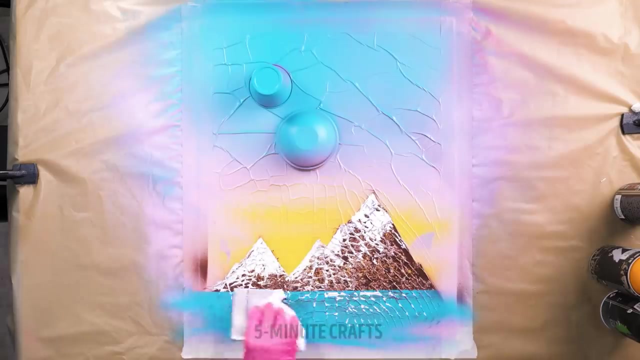 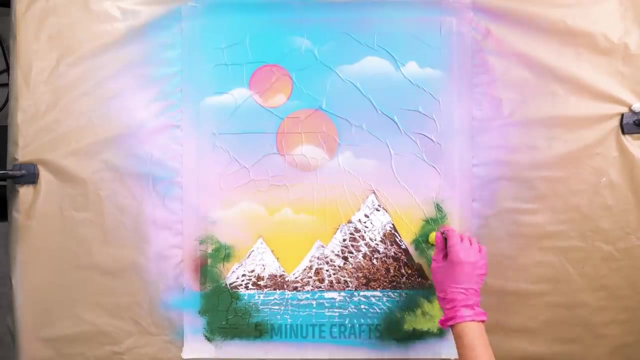 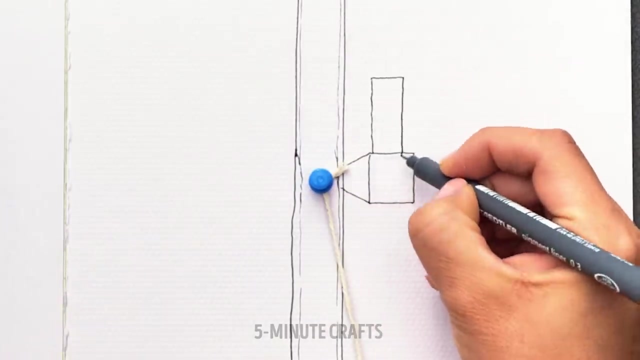 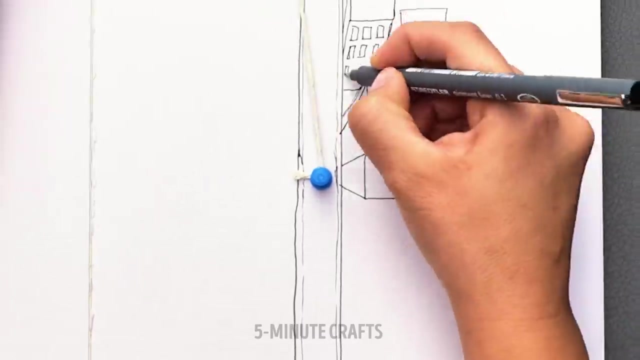 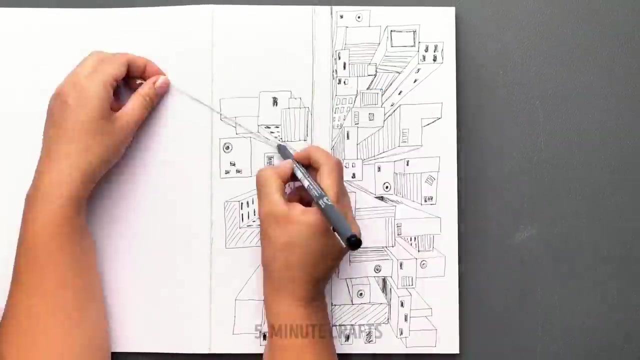 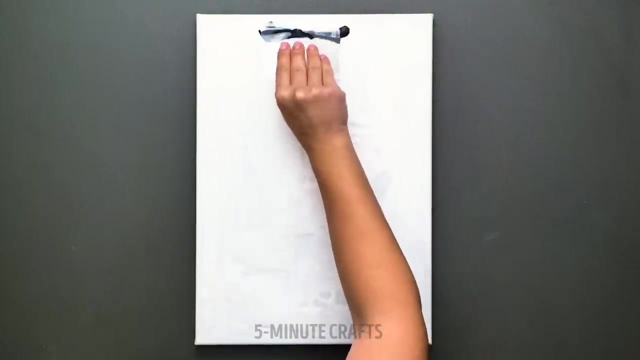 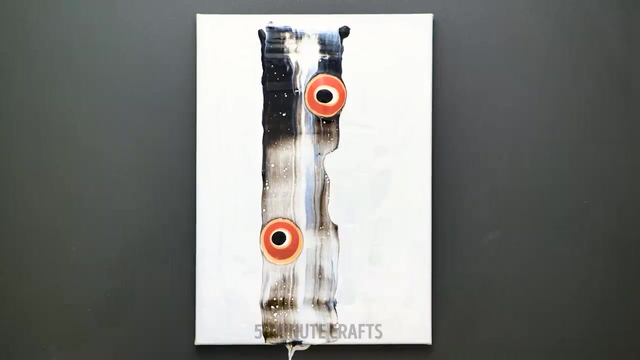 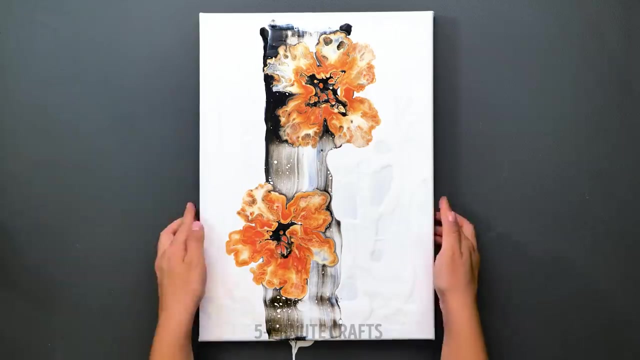 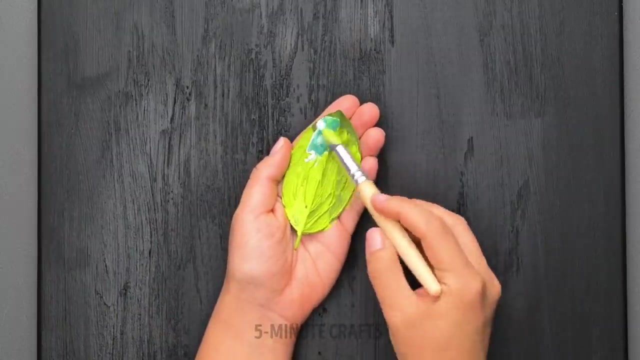 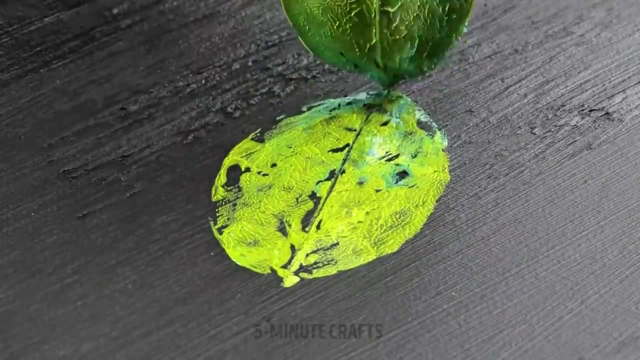 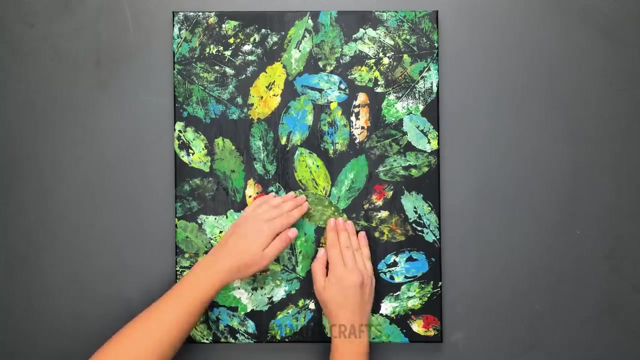 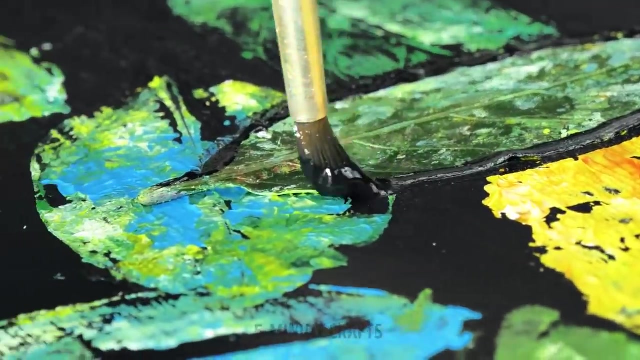 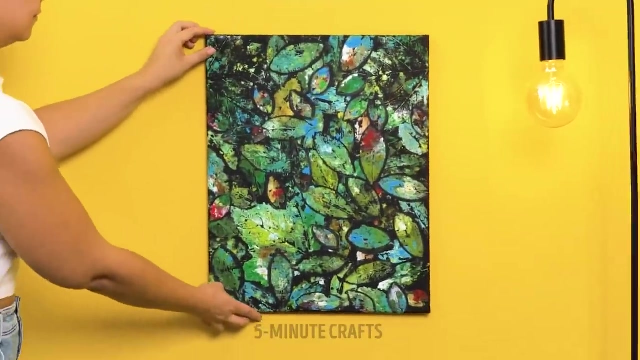 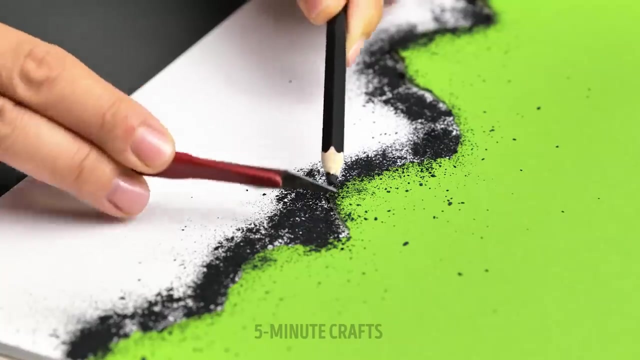 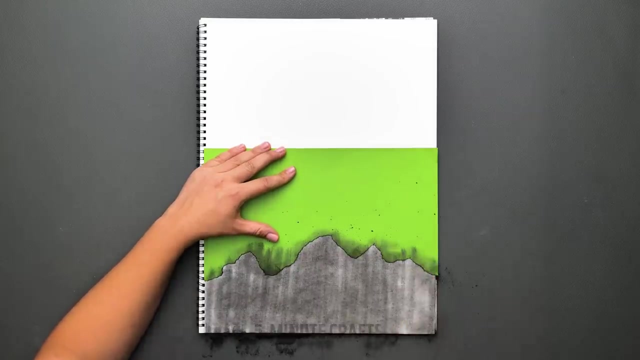 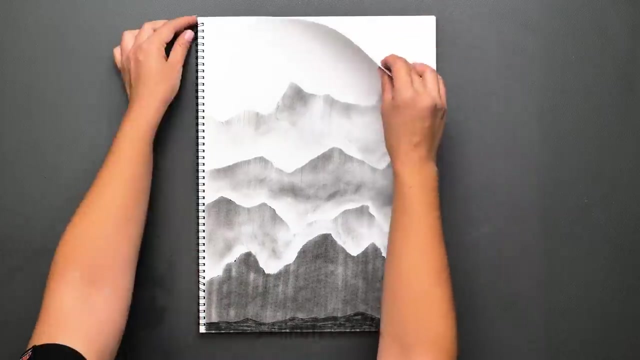 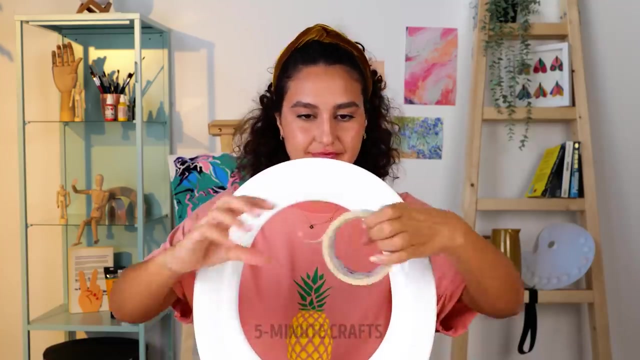 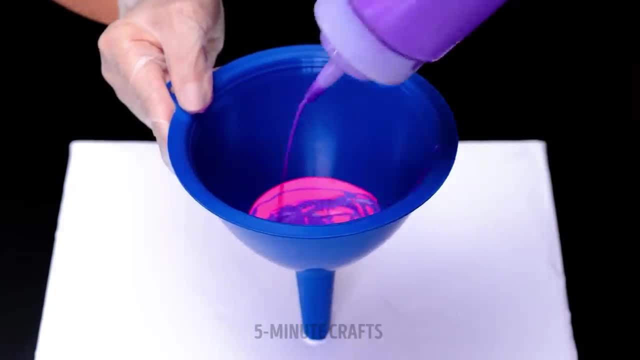 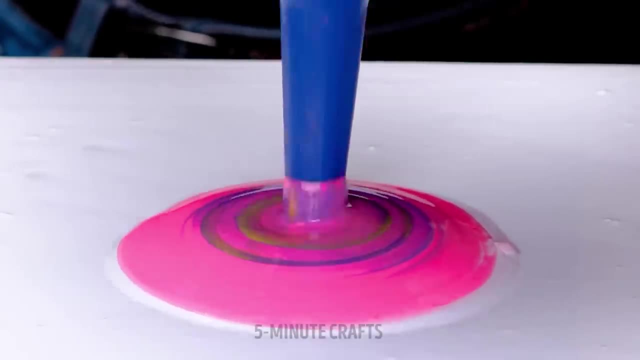 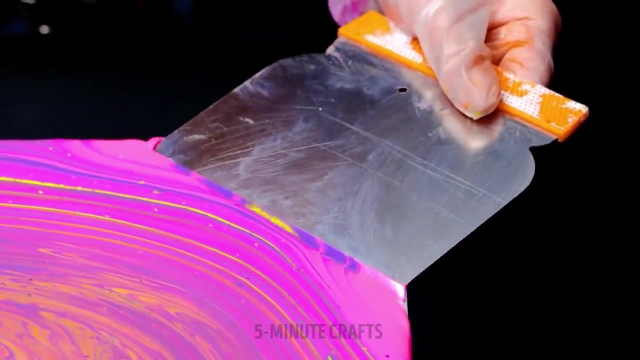 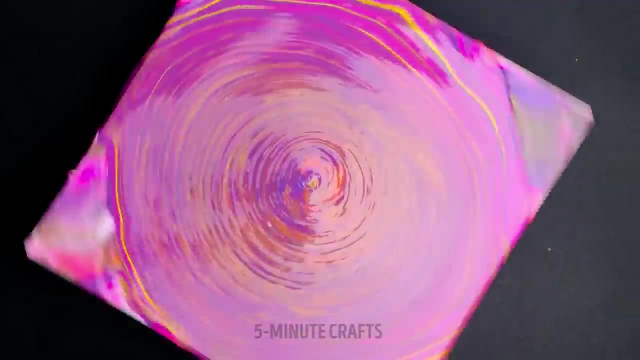 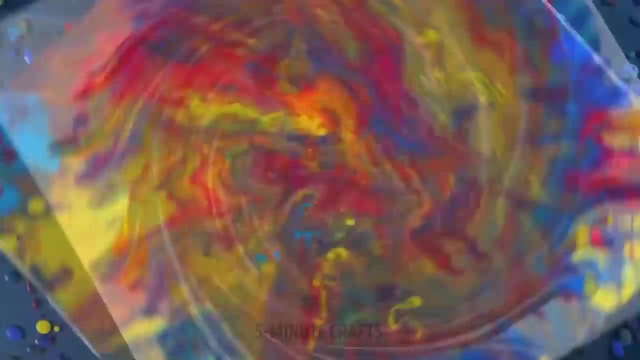 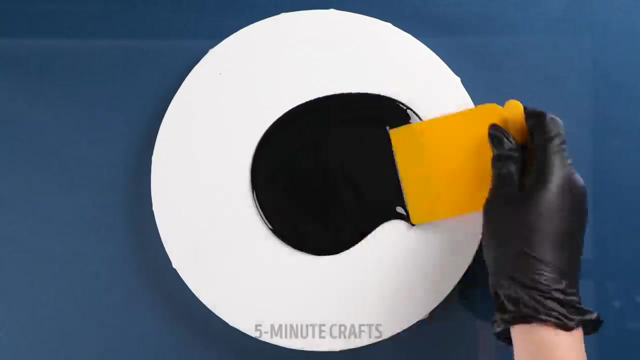 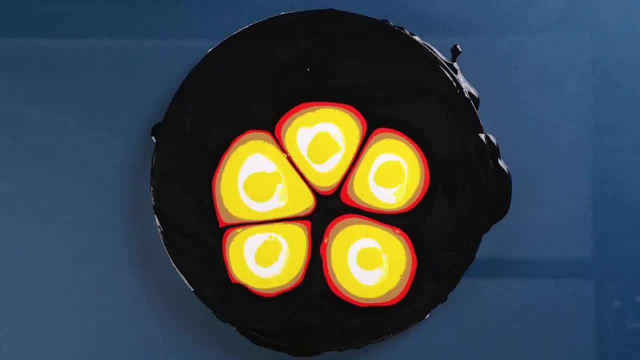 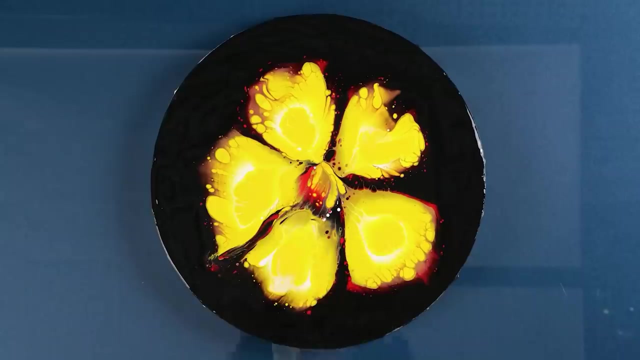 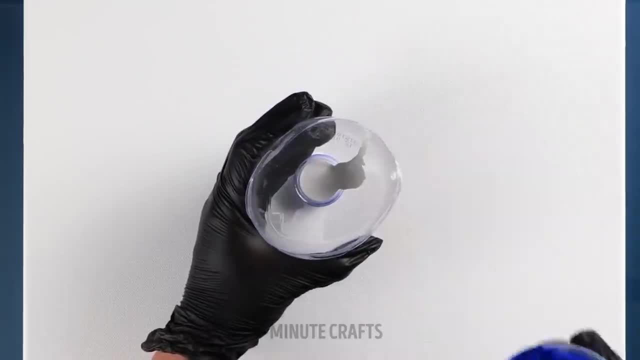 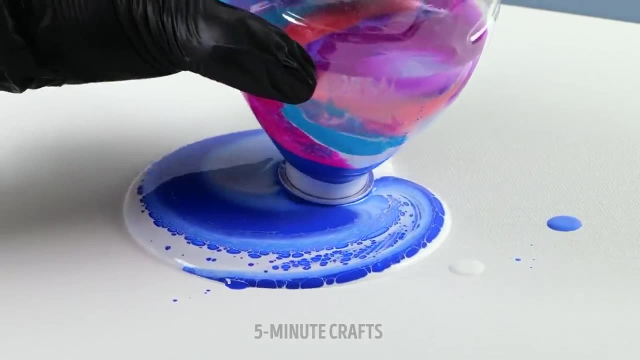 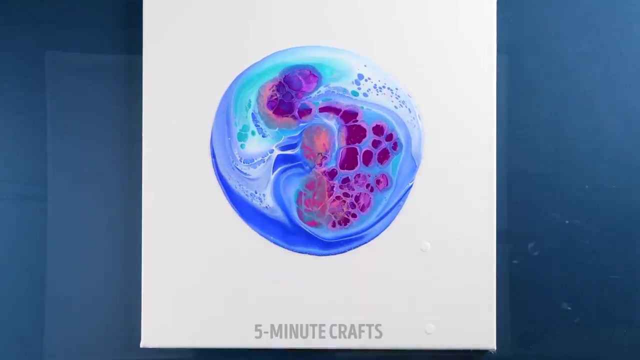 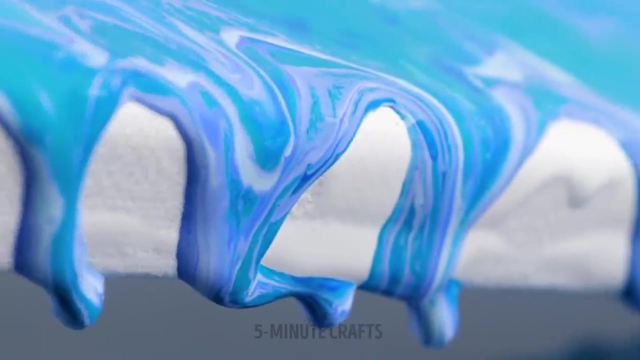 Such a short time in your life. All this hardship and convenience Makes it so hard to make it through. Are we missing out? Are we missing out, Baby? no, it's just a matter of time. We've thrown the tumble across the borderline, We're looking forward and we can't rewind. 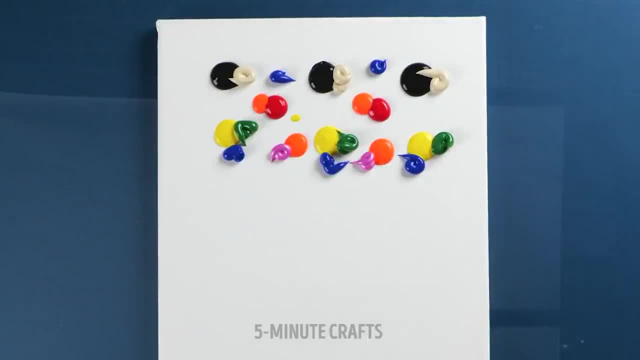 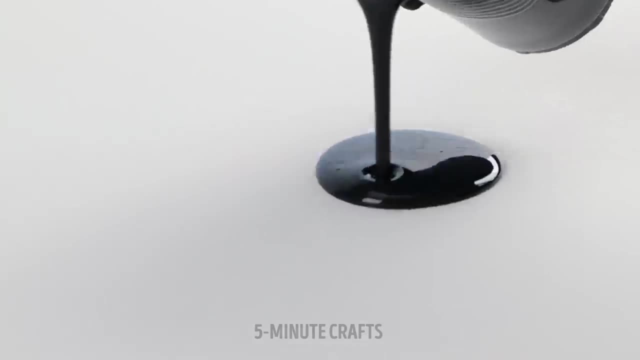 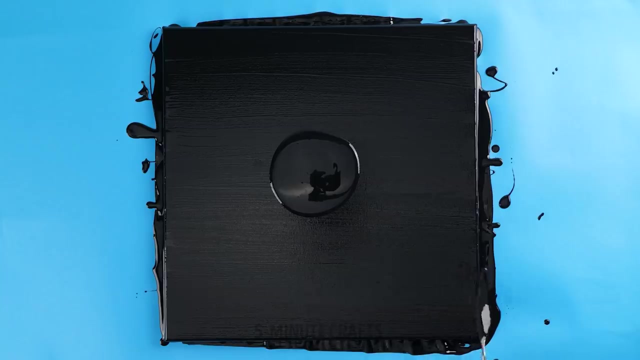 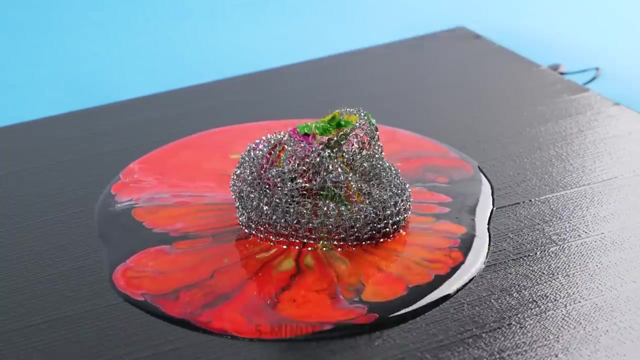 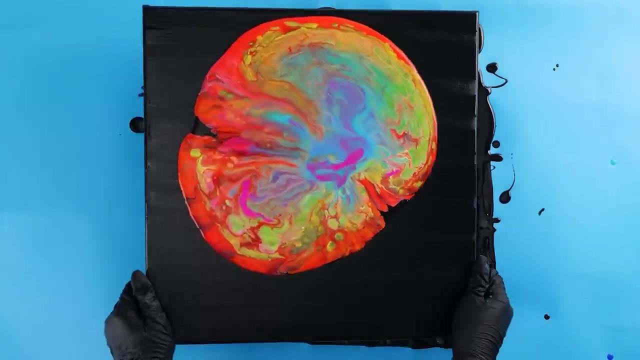 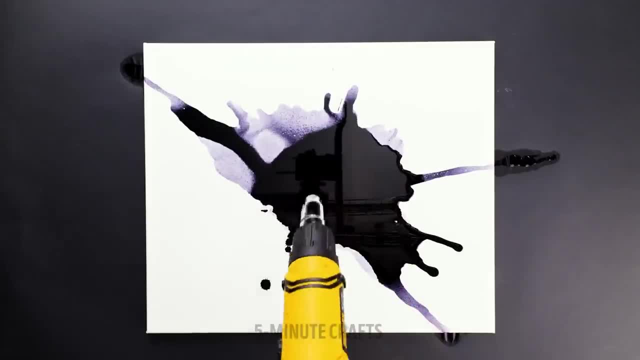 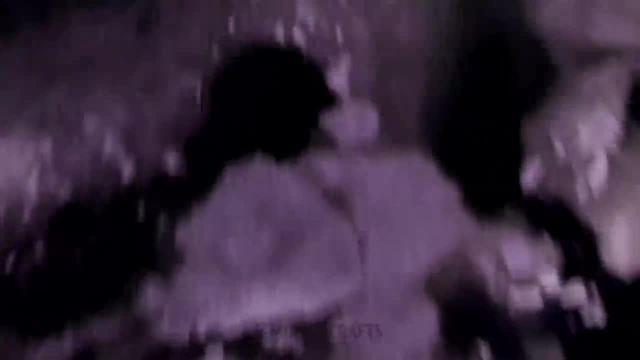 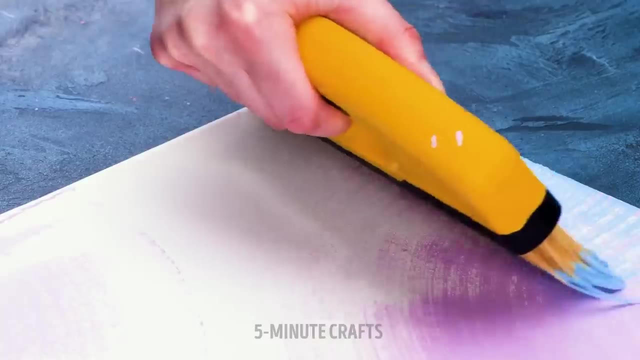 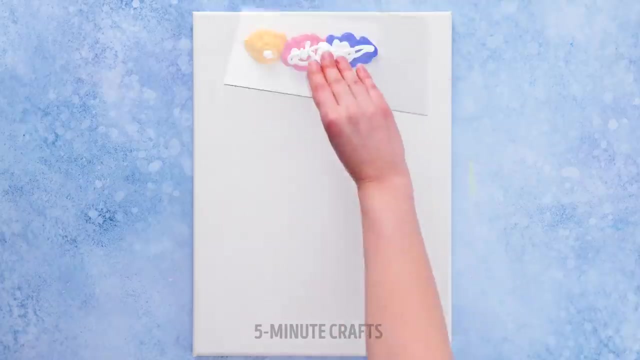 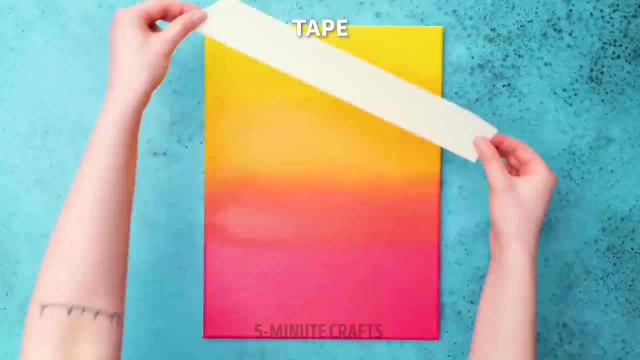 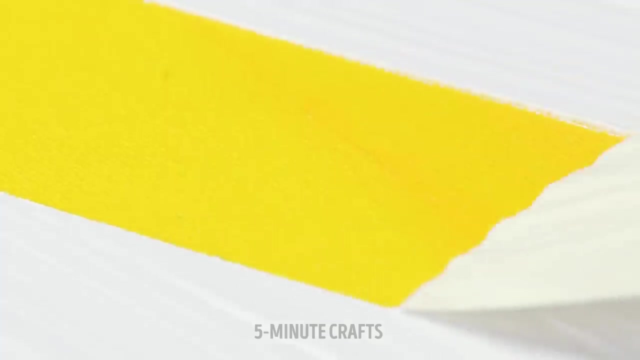 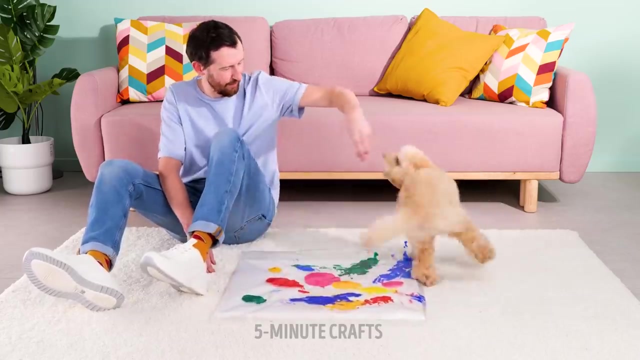 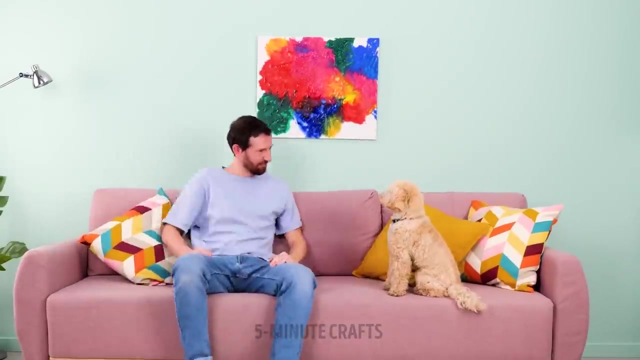 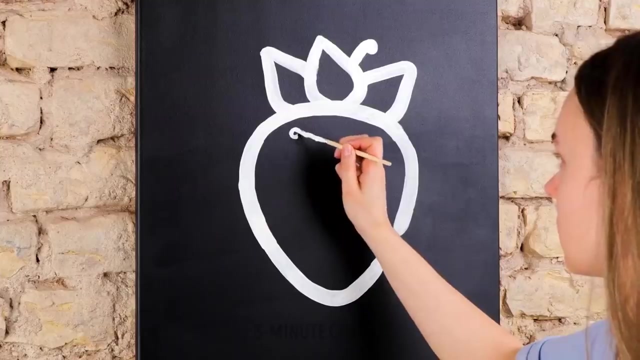 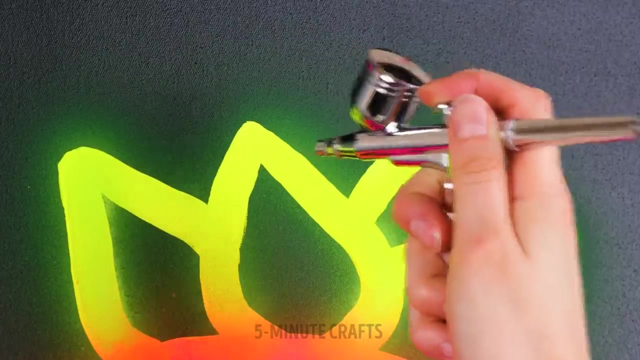 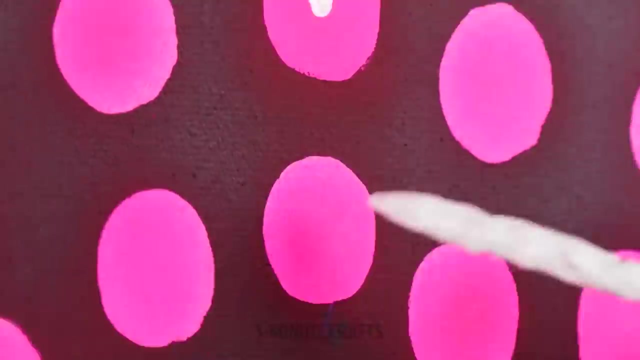 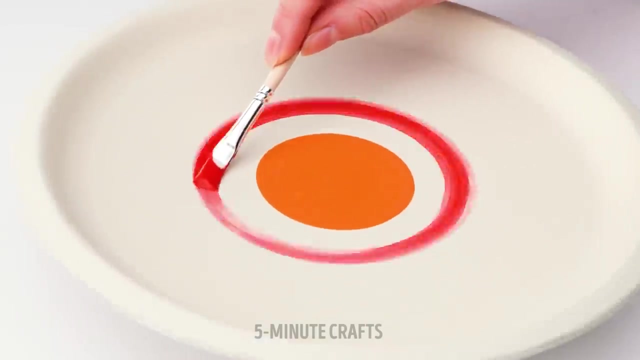 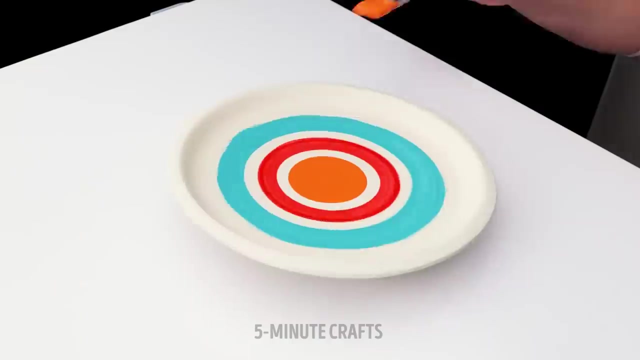 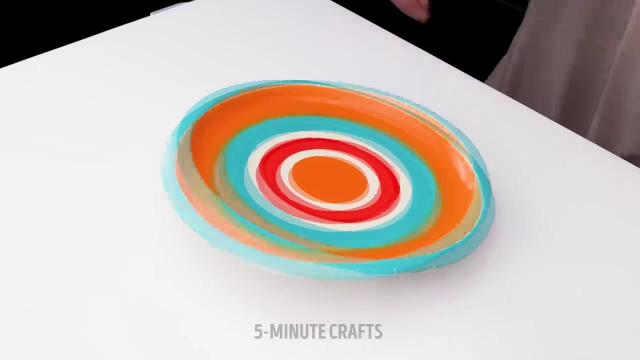 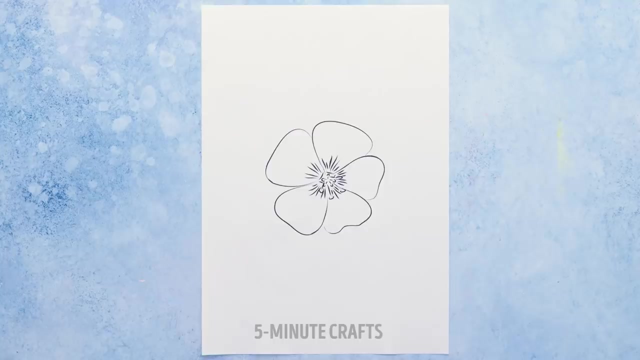 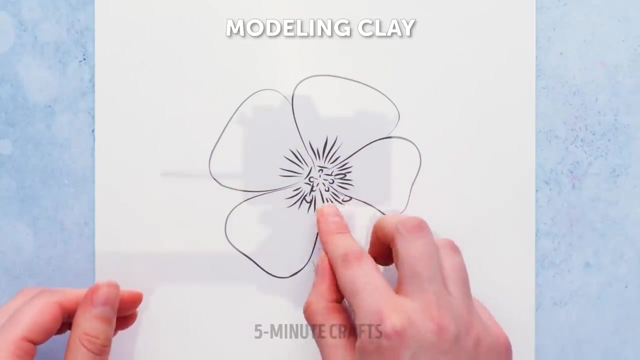 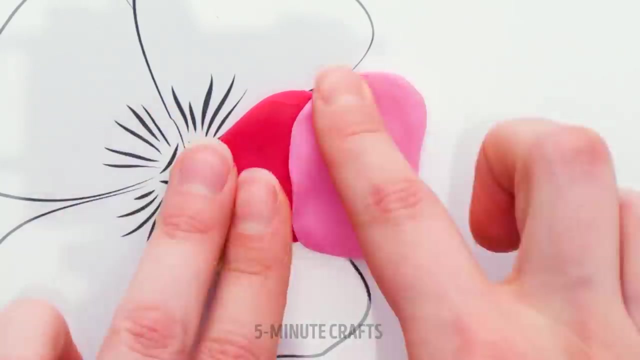 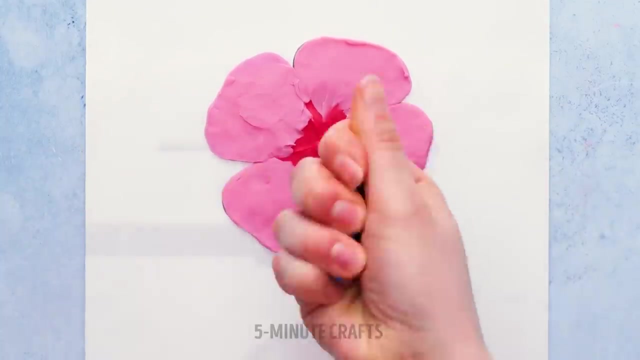 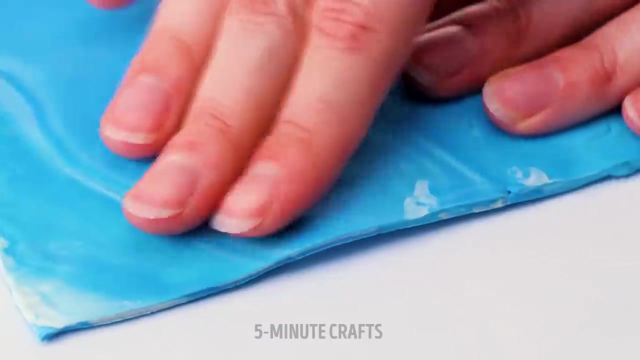 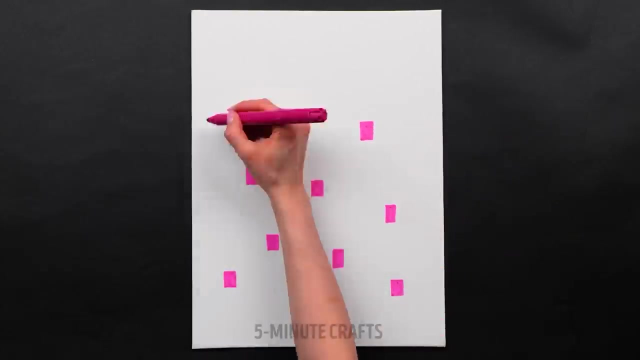 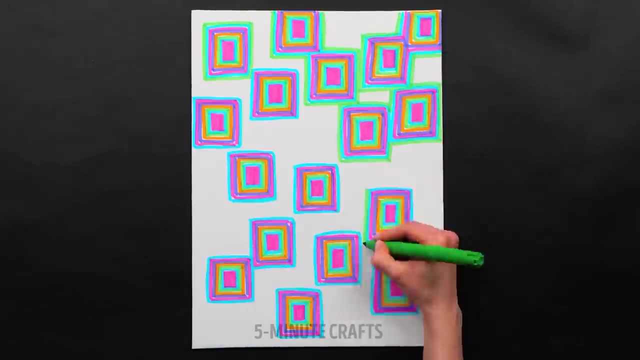 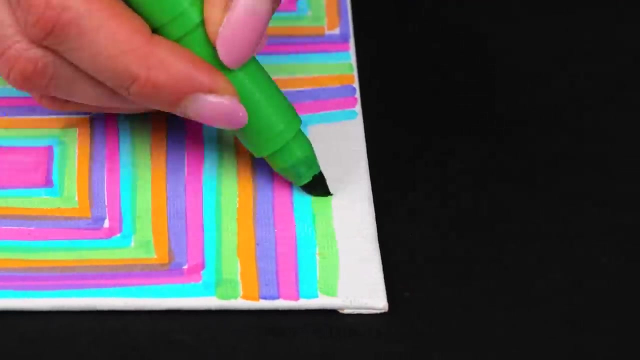 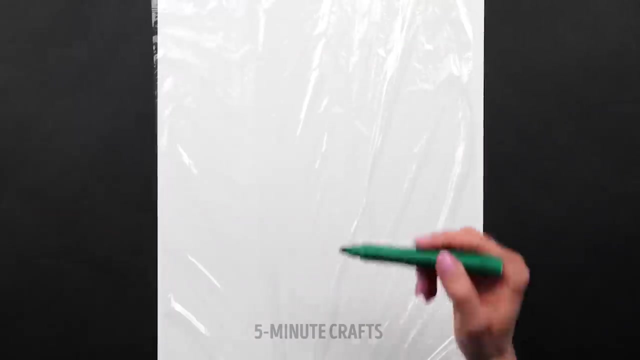 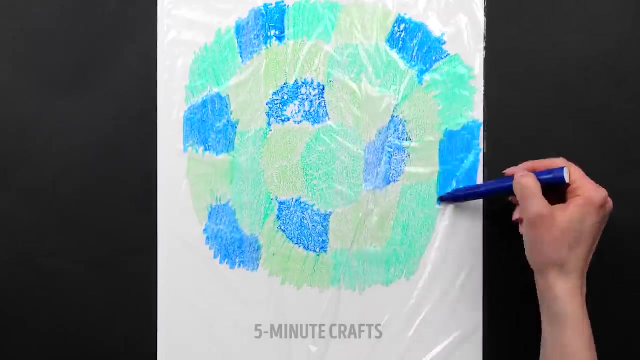 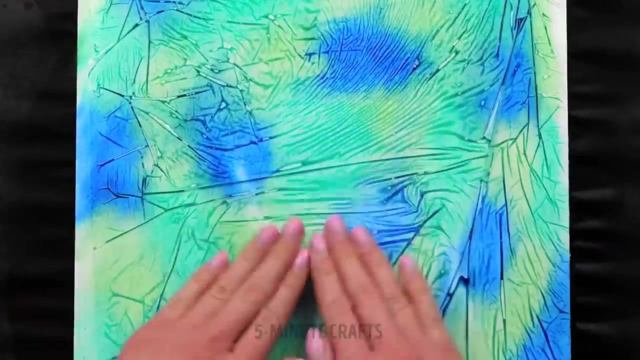 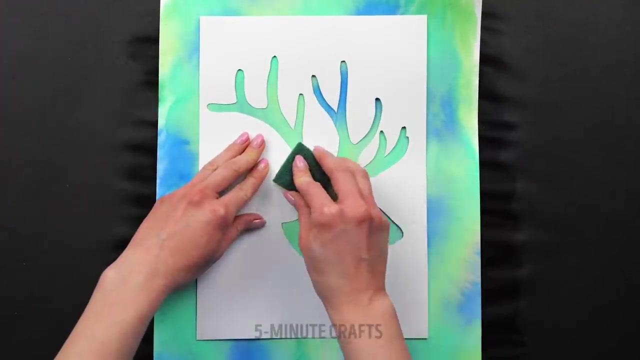 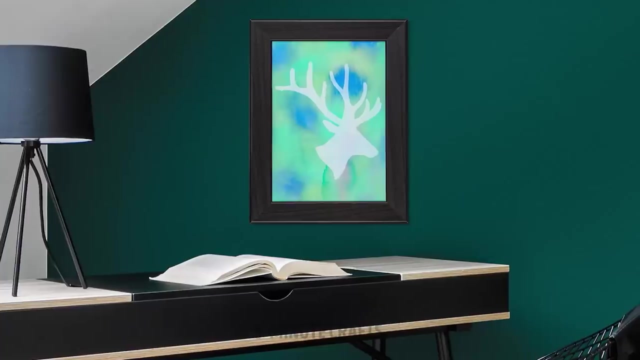 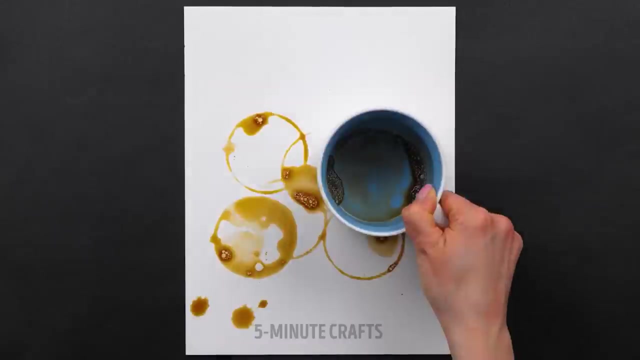 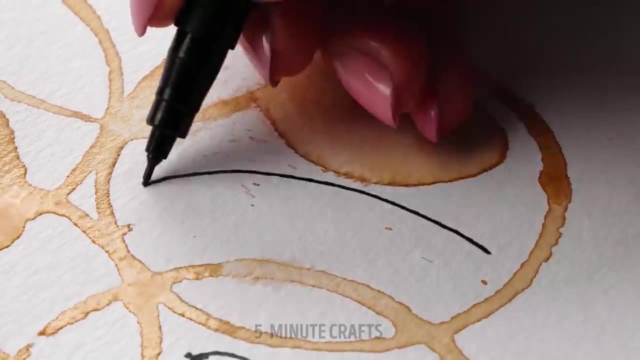 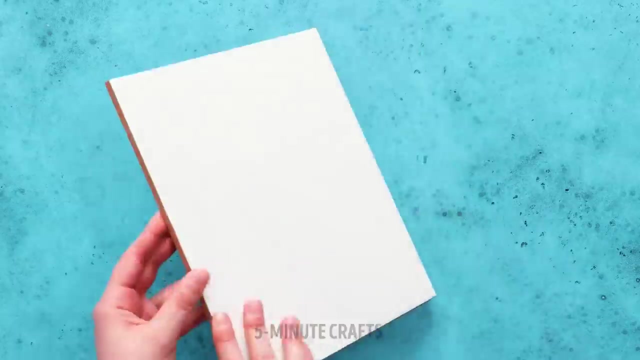 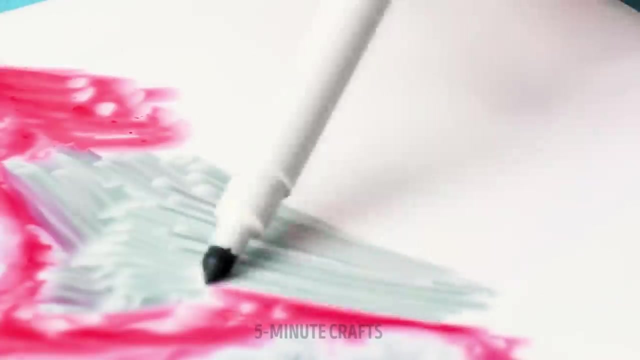 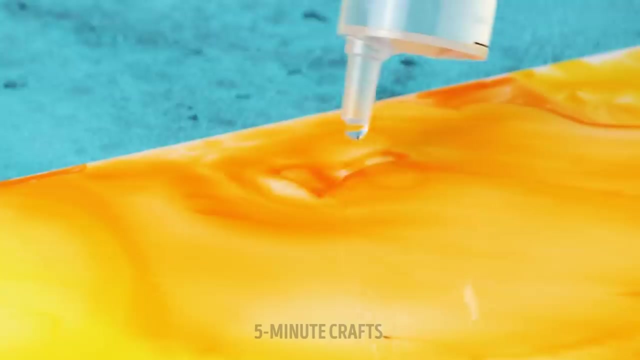 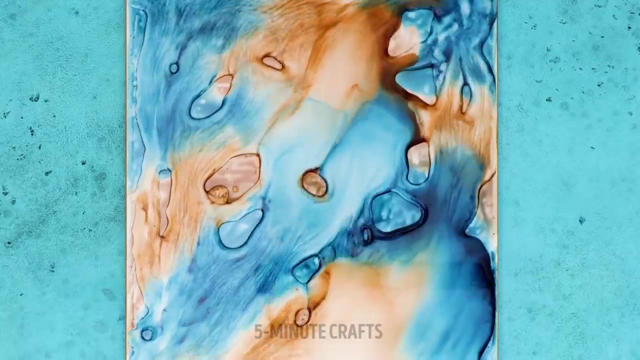 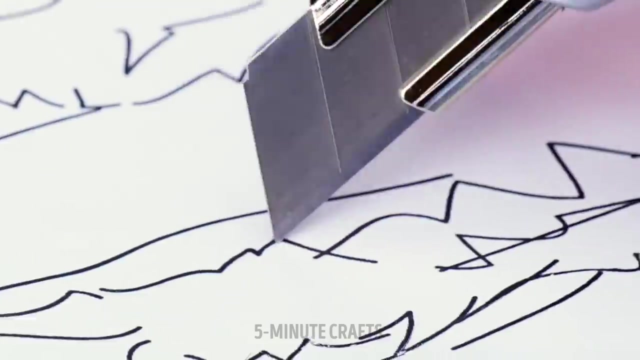 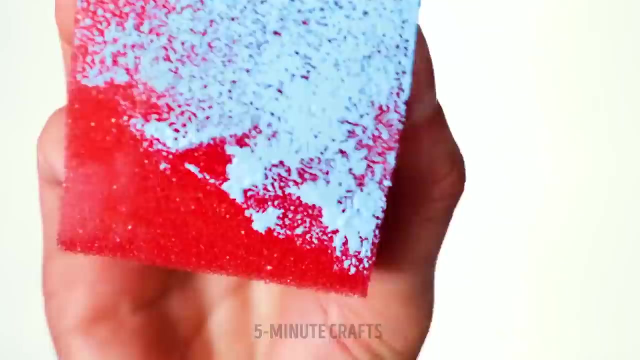 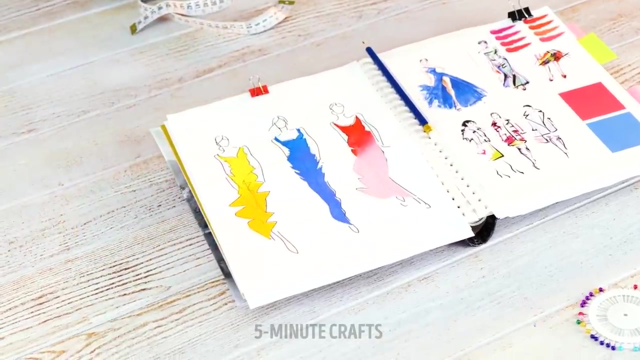 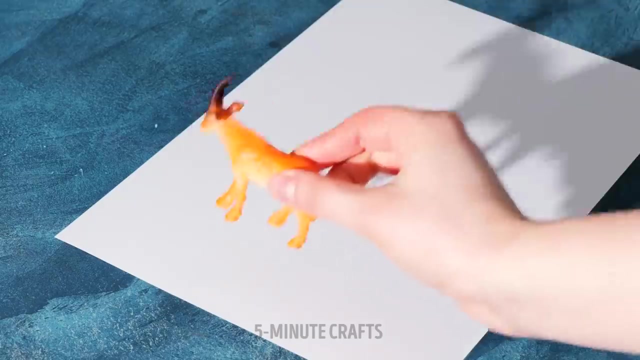 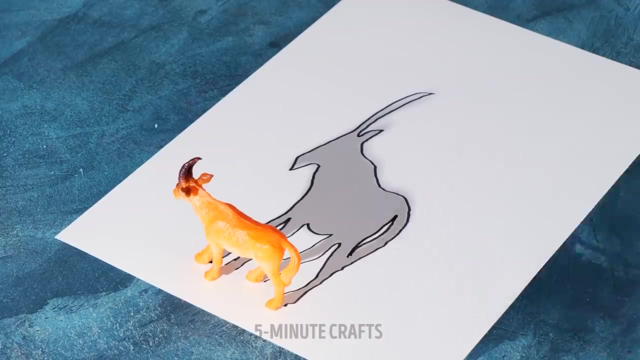 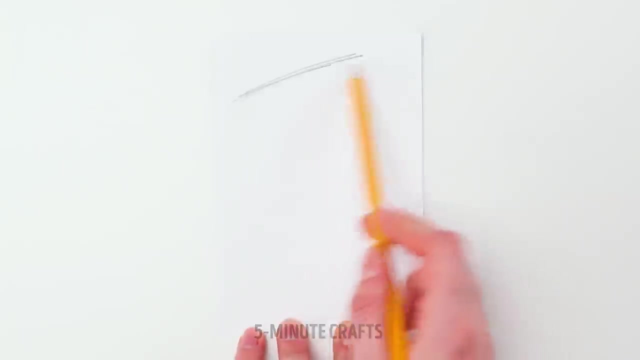 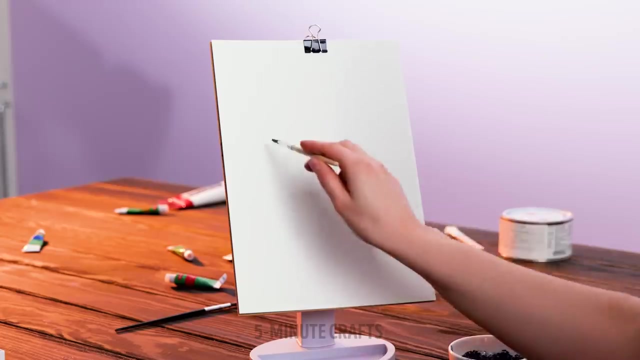 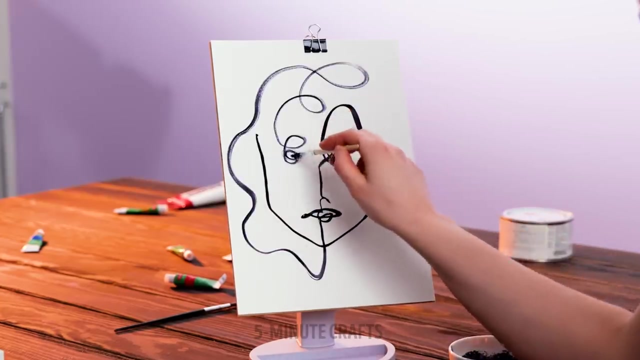